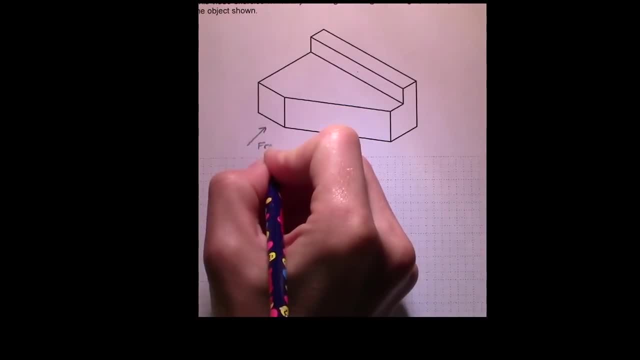 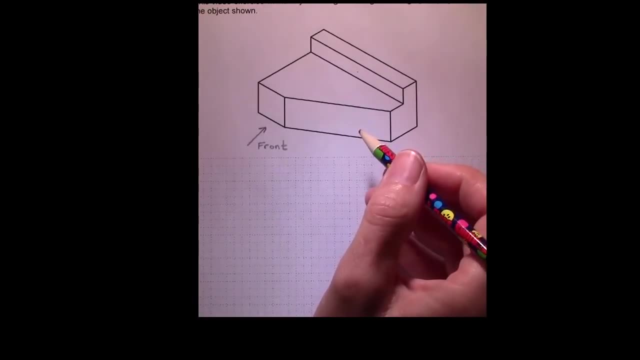 you know, tempted to call this your front view, because that's what looks like the front view. Now, in this case it's a little more complex, because the front view is really the view that shows the most about the object, but if you look in this direction, really all you see is a rectangle. So in reality, we should either choose this side. 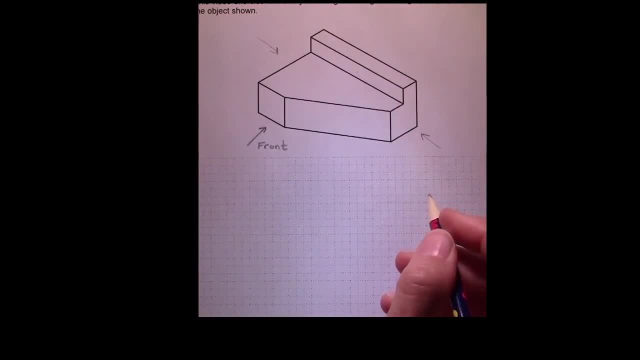 or or this to be our front view. However, we're just learning how to do orthographic projections and to choose either one of these views would be a lot of work, So I'm going to stick with the front view that's sort of shown in the figure, but just keep in mind this is not really the best front view. 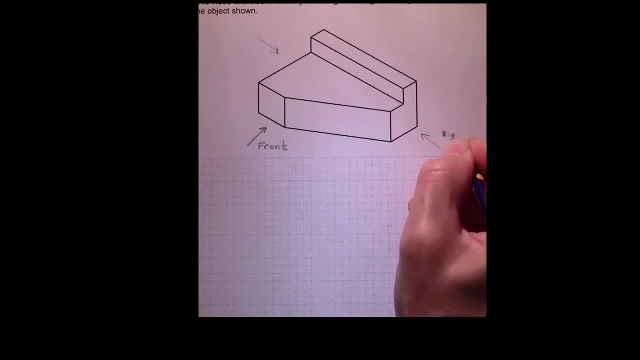 All right. so if this is our front view, then this is our right side view and this is our top view. All right, now to get a better handle on visualization. what I like to do is shade in all the surfaces that you're going to see. 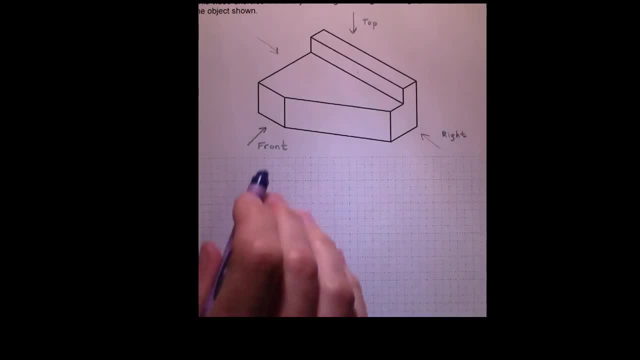 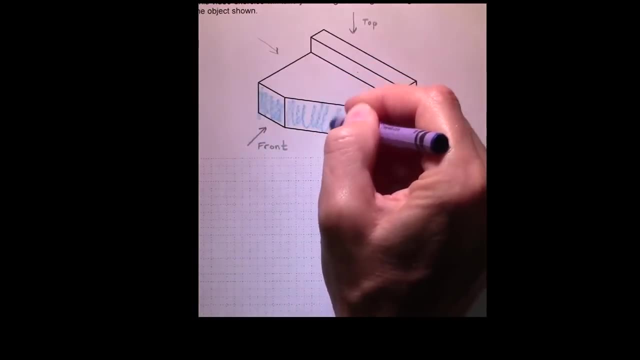 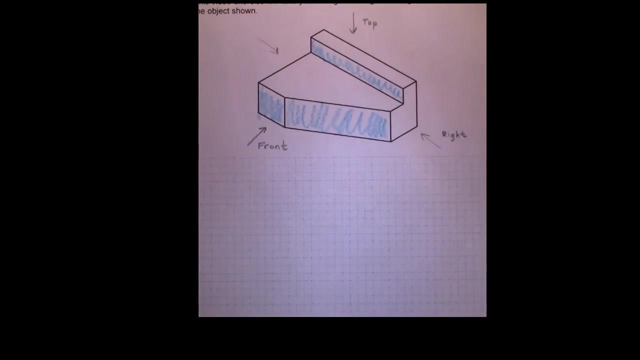 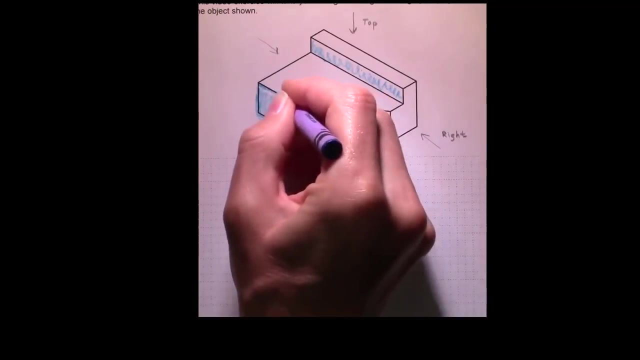 When you're constructing a particular view. so if we're doing the front view and we're looking this way, we would see this surface, that surface and that surface. So let's go ahead and draw that. So when we draw it we're going to see these shapes, right? 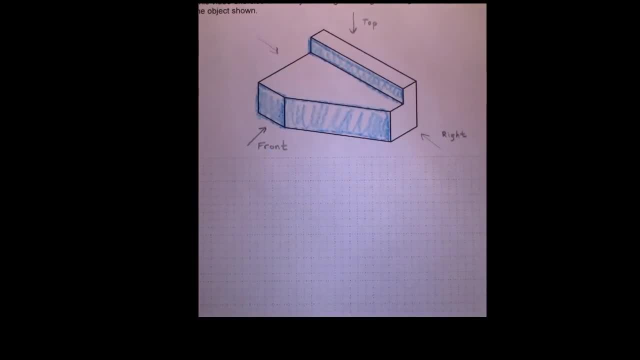 here. So that's what we should see in the front view. Now we don't have any dimensions, that's fine, we'll just kind of guess at the distances. All right, you can see that we have this rectangle here on the top, this here on the bottom, but we need to indicate where that surface starts to bend. 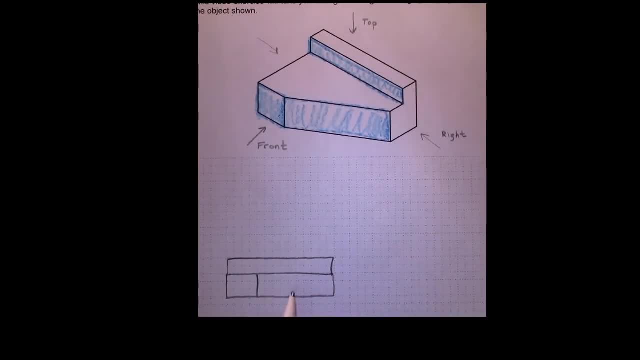 All right, so that's our front view. So you can see why this is not a terribly good front view, because it really doesn't show a lot about the object. All right, next we'll create the top view, and the top view is vertically aligned with the front view, So I'm going to draw projectors up. 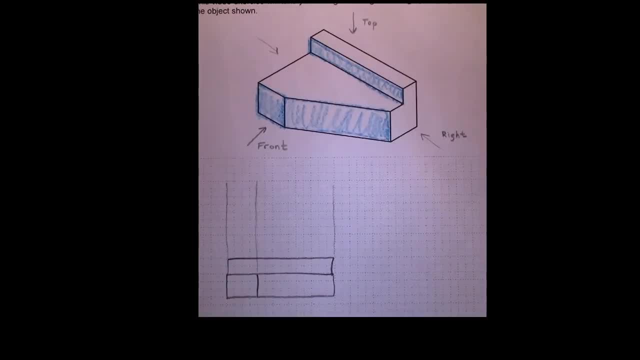 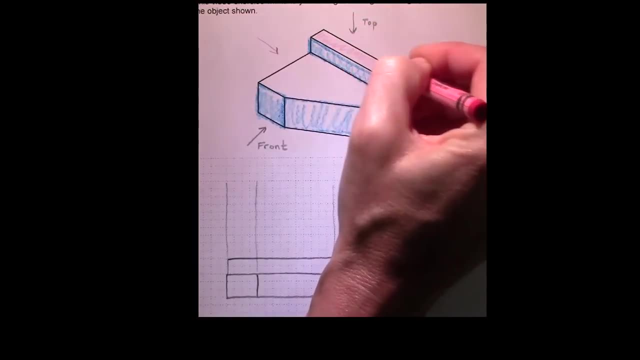 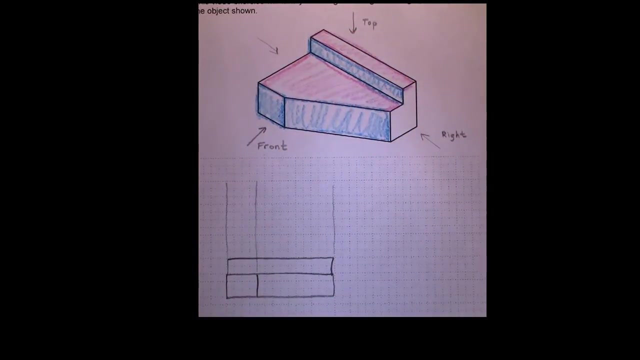 from every corner and edge of the front view and if we're doing the top view, we're going to be viewing down. this way, We'll see this surface here And this surface here, So the top view will have these shapes. All right. so I'm going to fill in this rectangle here. first, 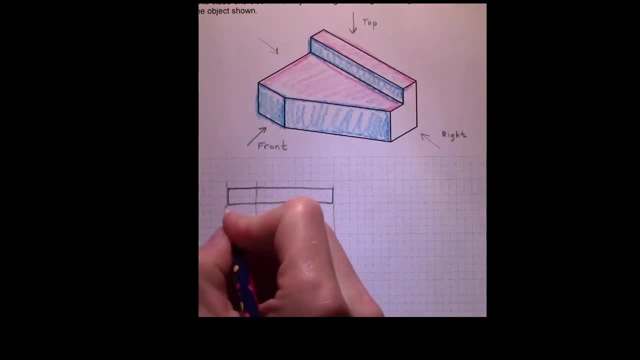 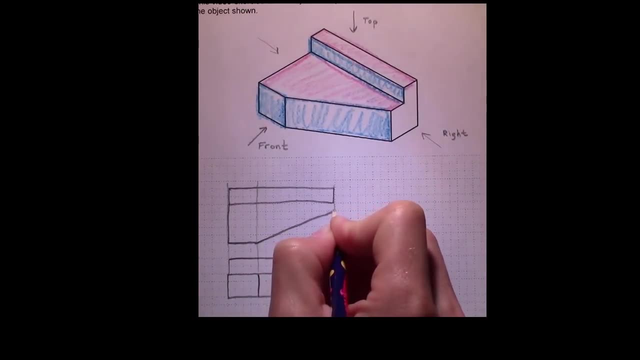 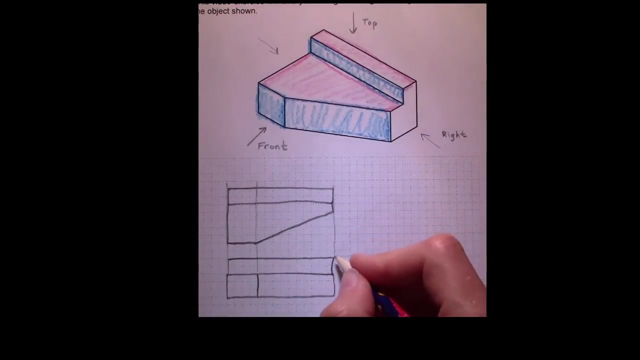 And then we have this shape. So we know, by the projector, this is the where it starts to angle back, and there we go. so that's the top view. the right side view is going to be horizontally aligned with the front view, and then we're going to create a 45 degree angle projector and project over and down from. 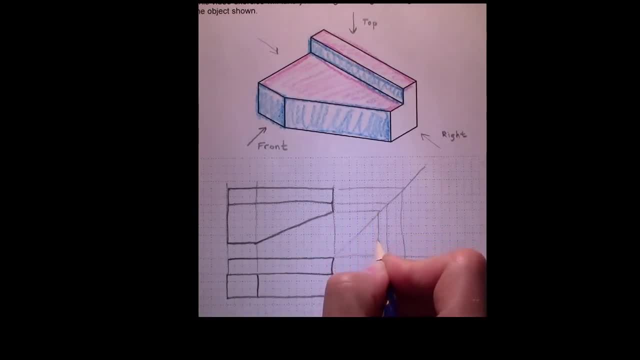 the top view and this gives us a nice little area where our right side view is going to go. so if we shade in our surfaces, we're going to be viewing this way, we're going to see that shape and we're also going to see some of the 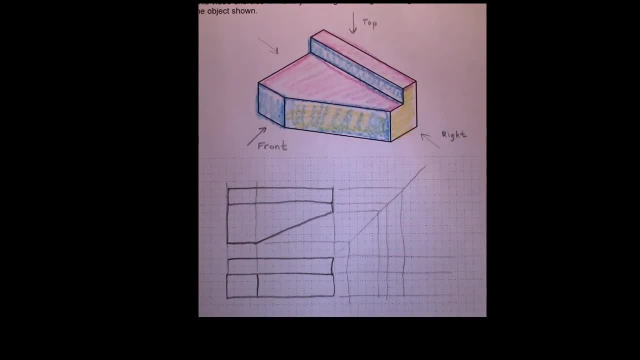 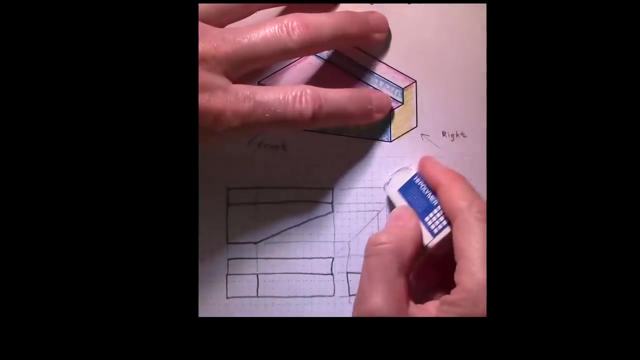 angled surface. all right. so let's draw this shape in first, and the projectors will guide you, and then the angled surface. All right, so that's our right side view. The last thing we need to do is to erase our projectors, or, if you're in a CAD program, just turn that layer. 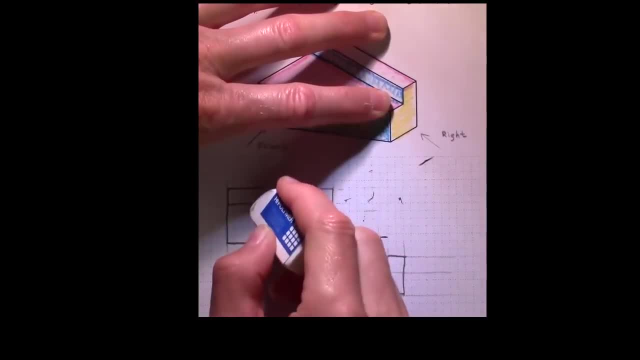 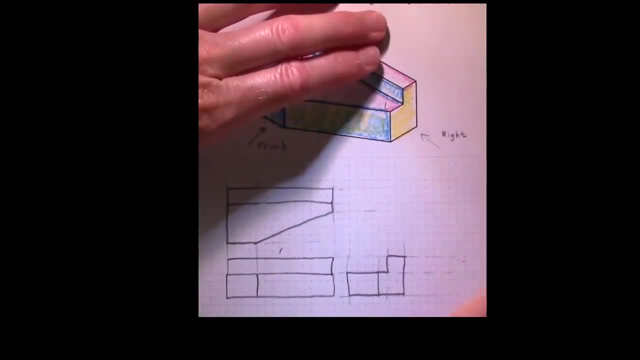 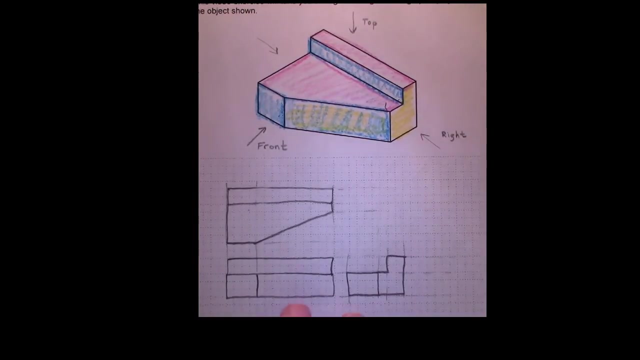 off so that we don't get confused with what our visible lines are and what our projectors are. And my suggestion is, when you're sketching these orthographic projections, if you're just beginning, definitely use a pencil, because you're going to be erasing a lot.